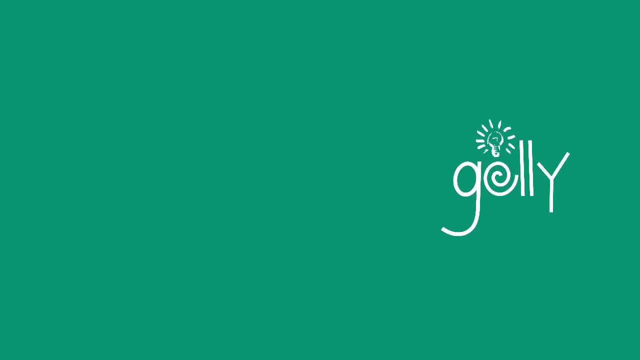 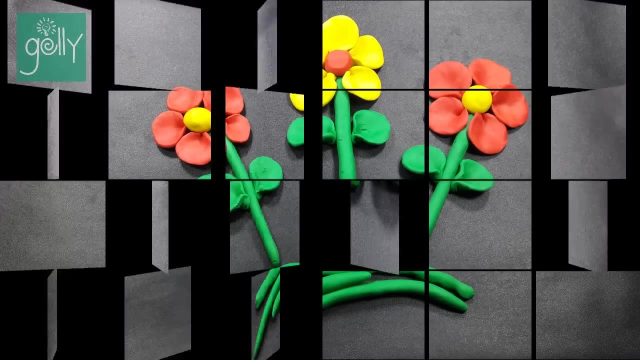 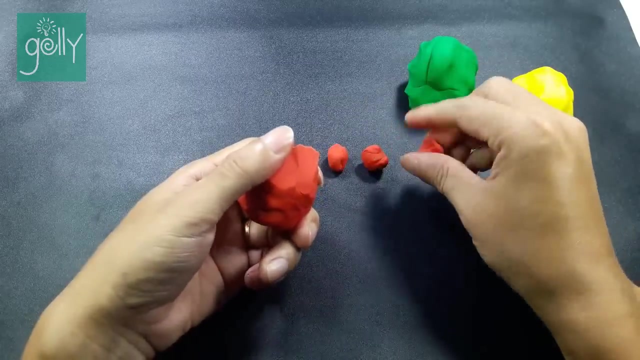 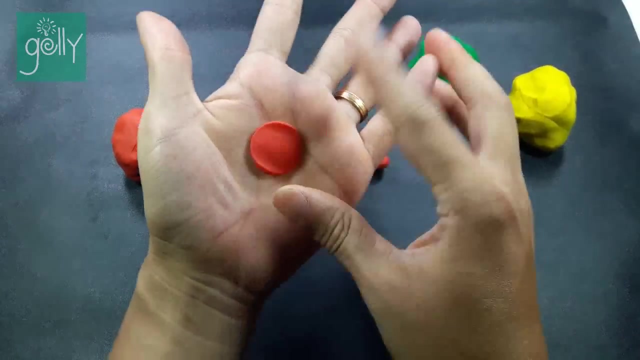 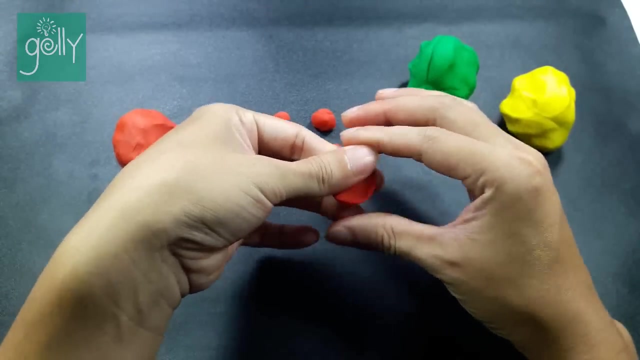 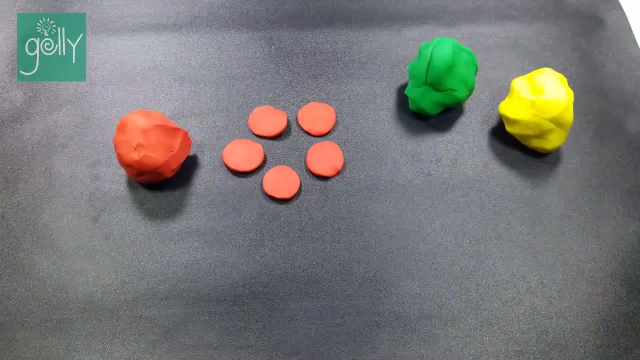 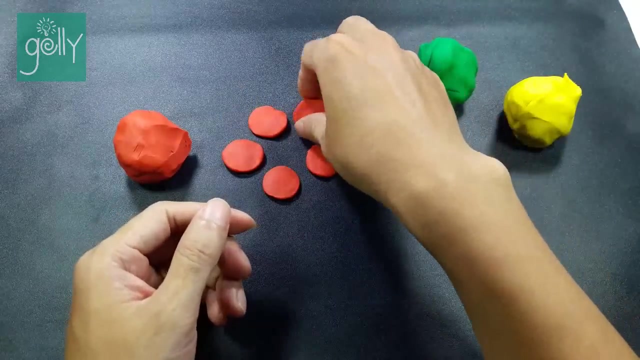 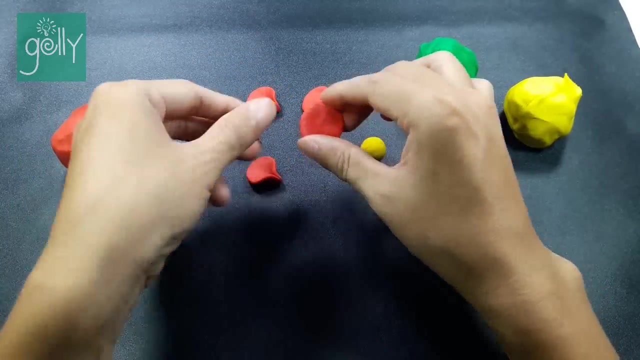 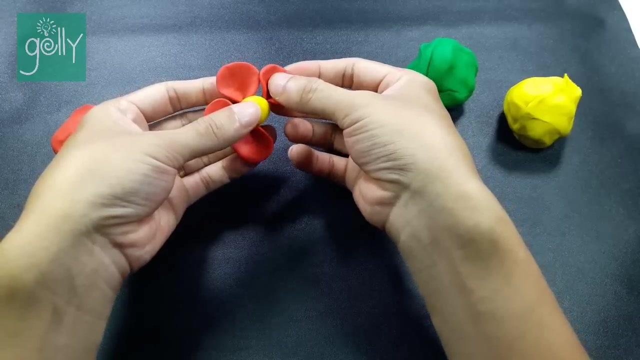 Twinkle, twinkle little star. How I wonder what you are, Up above the world, so high Like a diamond in the sky. Twinkle, twinkle little star. How I wonder what you are When the blazing sun is gone, When the nothing shines upon. 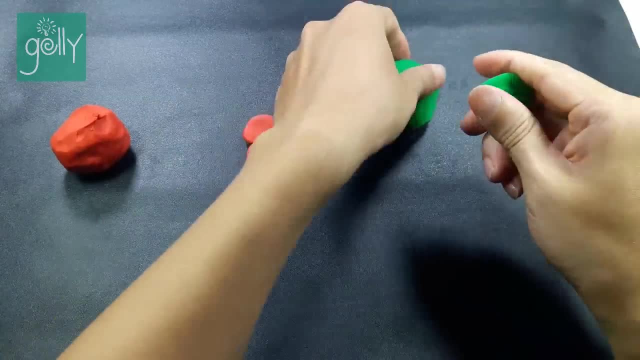 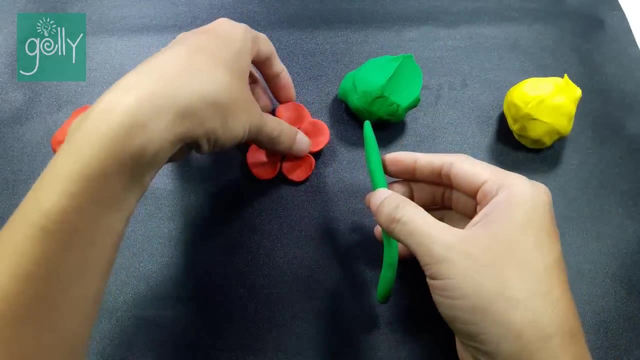 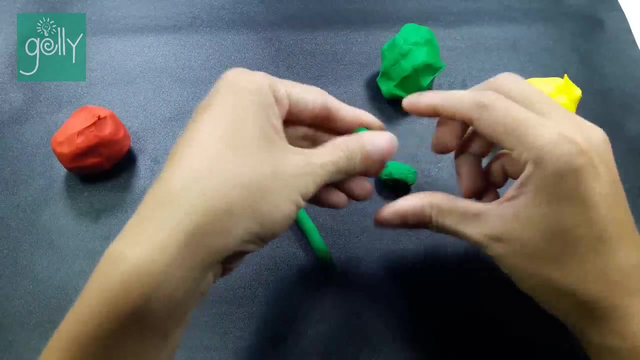 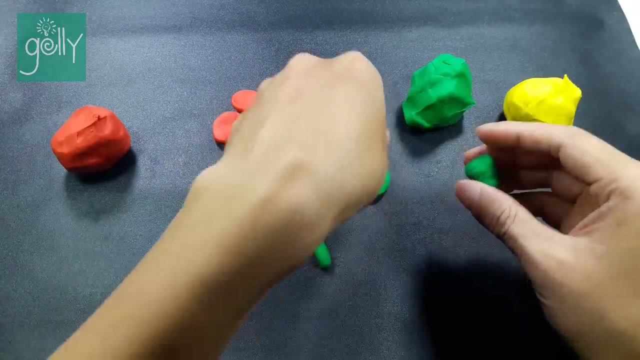 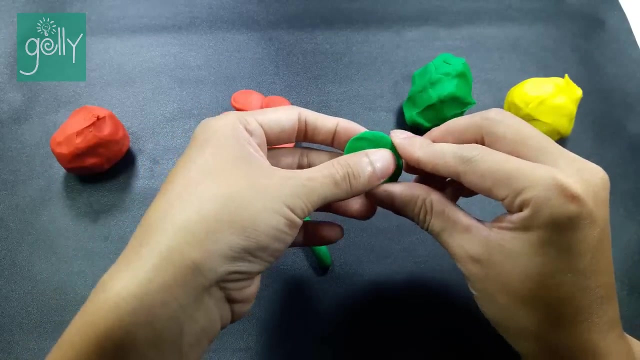 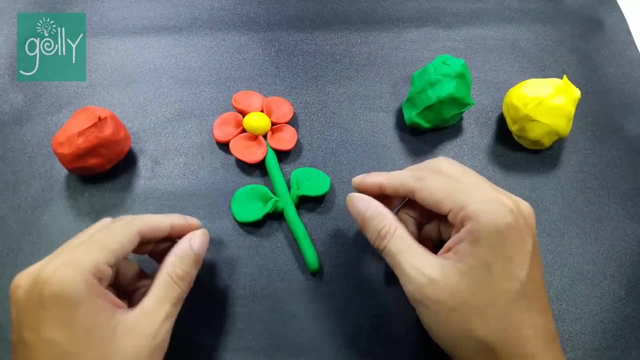 When you show your little light Twinkle twinkle all the night. Twinkle twinkle, little star. How I wonder what you are. Twinkle twinkle, little star, How I wonder what you are, Up above the world so high Like a diamond in the sky. 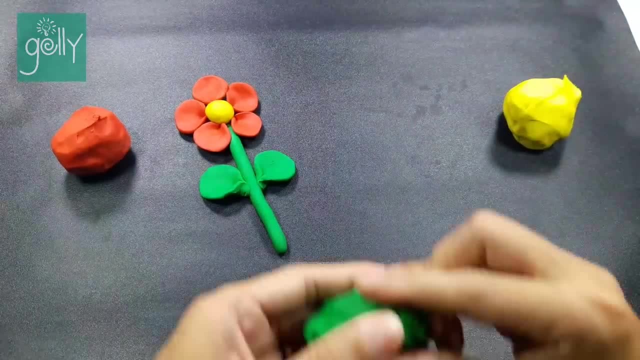 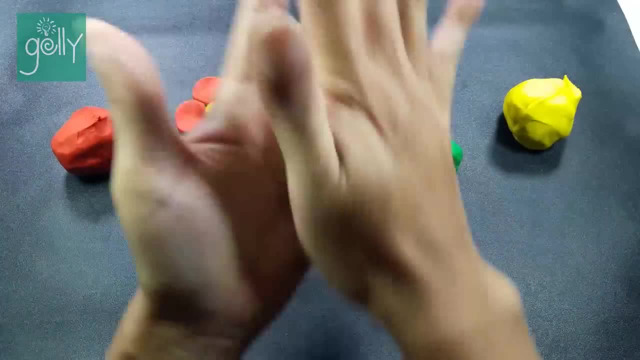 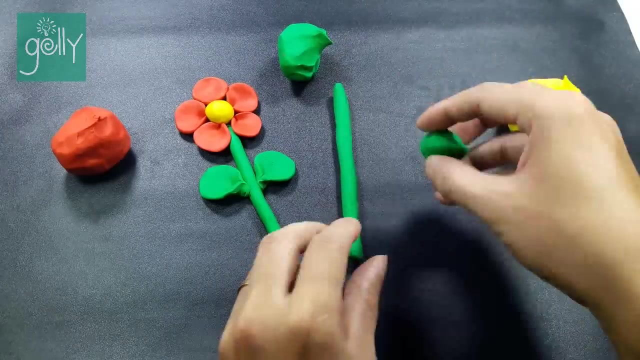 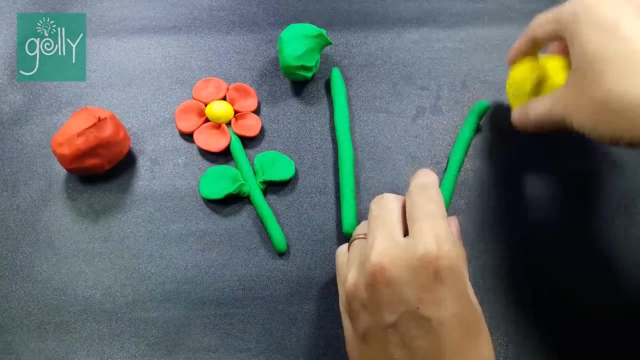 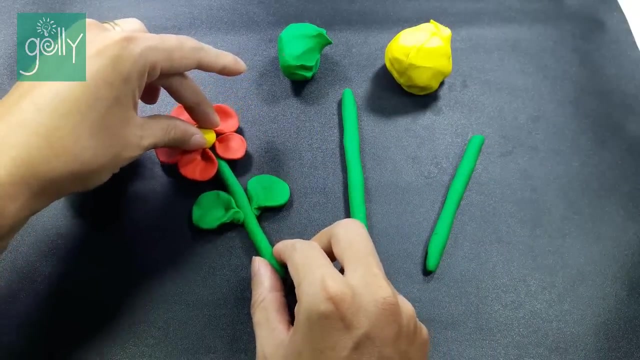 Twinkle, twinkle little star. How I wonder what you are Up below the world, so high Like a diamond in the sky. Twinkle, twinkle little star. How I wonder what you are Up above the world so high Like a diamond in the sky.